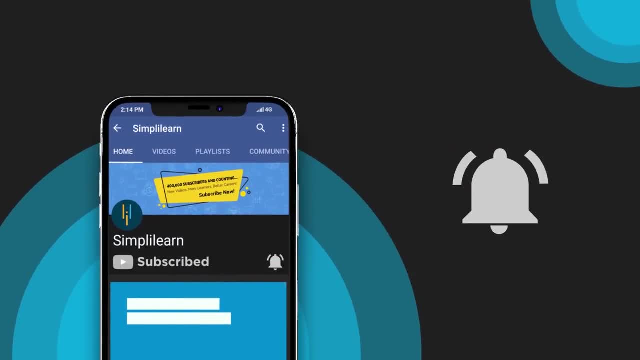 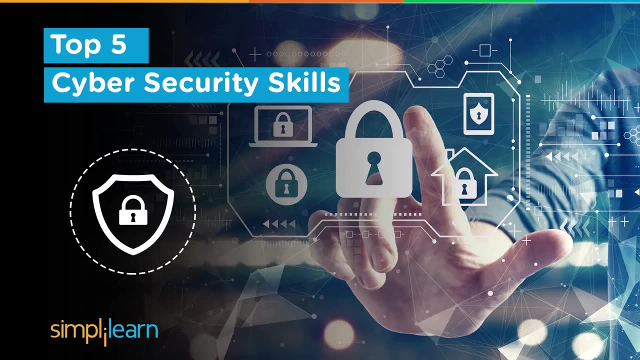 With businesses moving online and shifting to cloud storage, currently the demand for cybersecurity is at its peak. With that comes a high demand for cybersecurity experts who can safeguard digital data. On that note, hey guys, welcome to yet another exciting video. by Simply Learn. In this video, we bring you the top 5 cybersecurity skills. 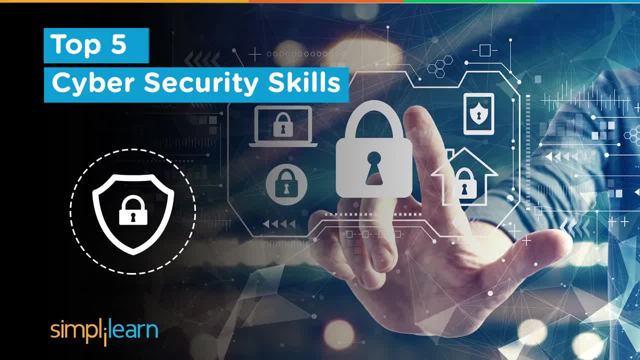 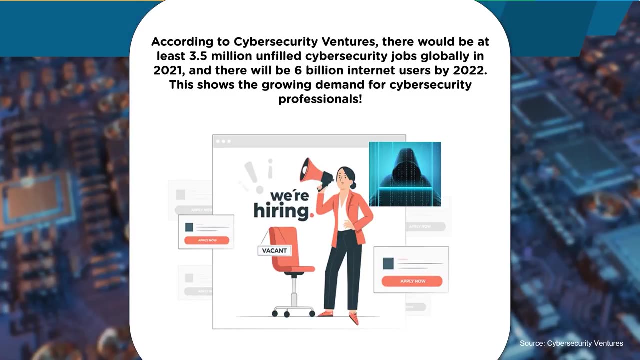 But before we begin, if you are new here and haven't subscribed already, make sure to hit the subscribe button and the bell icon for interesting tech videos every day. So let's get started. According to Cybercrime magazine, by Cybersecurity Ventures, globally there would be nearly 3.5. 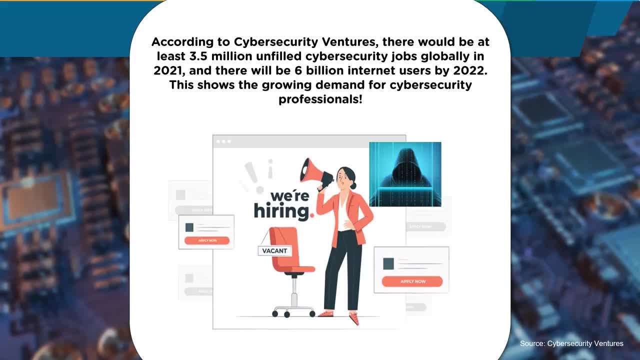 million unfilled cybersecurity jobs by 2021 and the number of internet users will hit a whopping 6 billion by 2022. These numbers speak volumes and this shows the growing demand for cybersecurity professionals across the globe. Now that you know the high demand, 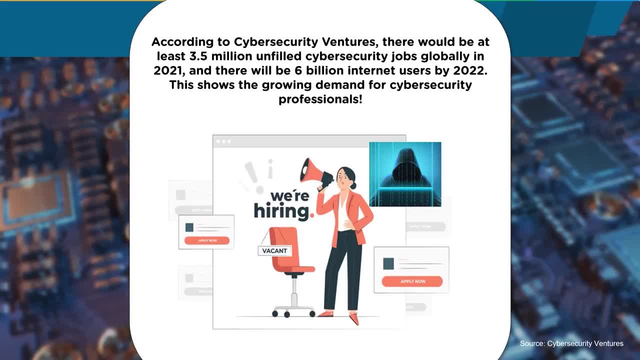 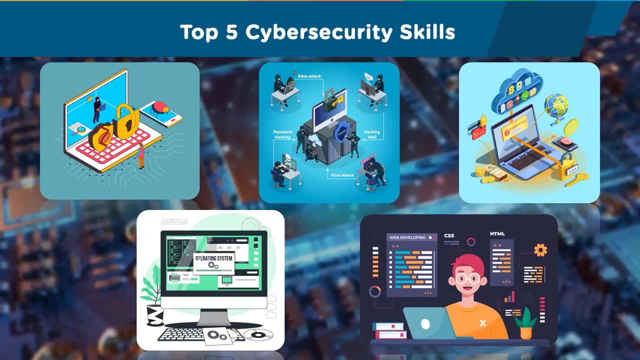 for cybersecurity professionals. let us help you start your cybersecurity career by bagging the right skill set. Many of you out there might be waiting to become a cybersecurity professional, but are unsure of how to go about it and what skills you would need to get a cybersecurity job. 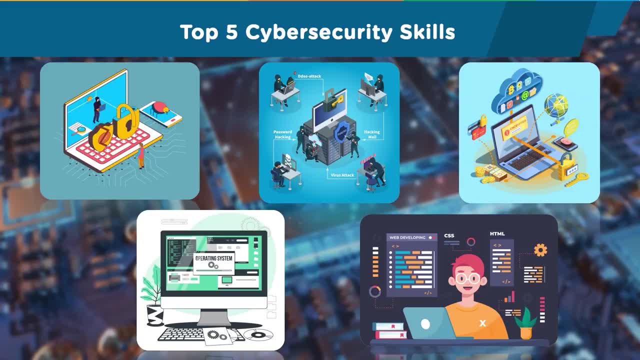 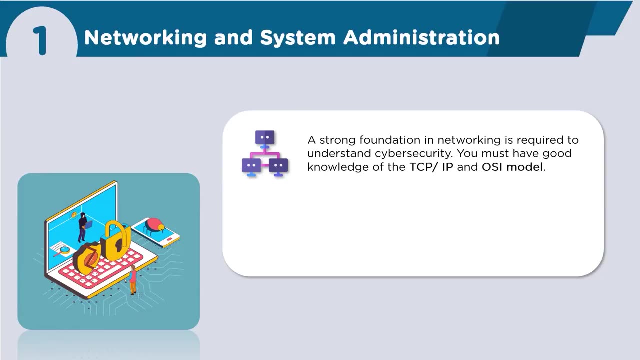 Not to worry, we are here to help you with that. After extensive research, we have come up with the top 5 skills that will help you get into the field of cybersecurity. Let's have a look at these skills individually. First, we have networking and system administration. 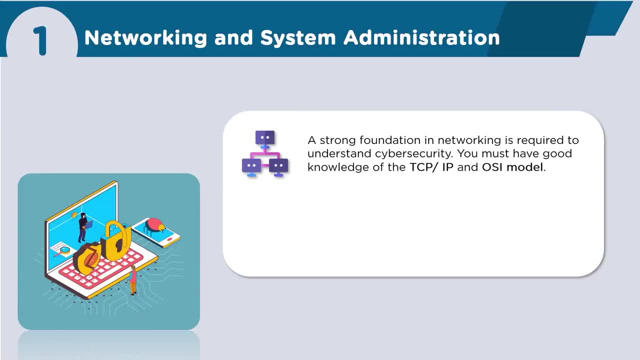 The number one skill you need to have to enter the field of cybersecurity is computer networking. Networking is the backbone of the internet. It is imperative that you have an in-depth understanding of networking to start a career in cybersecurity. A network is a group of 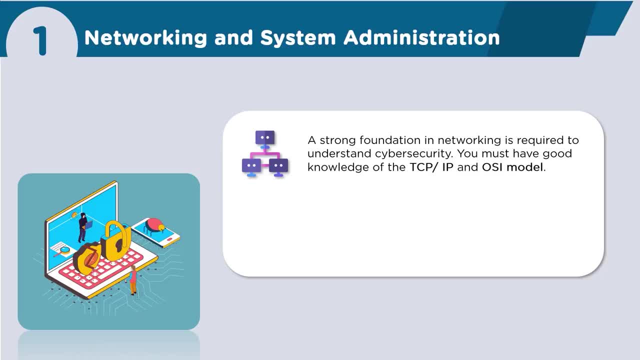 interconnected devices, and networking is the art of understanding how data is sent, transmitted and received amongst these devices. You need to know various routing protocols. The TCP, IP and OSI models govern networking. The OSI model is comparatively newer. Basically, in these models, all the protocols are grouped into layers and work together to help you receive. 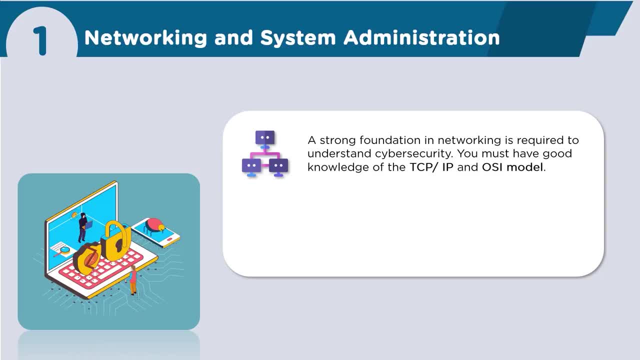 data on your device sent from a server. Learning networking will help you understand the technical aspects of data transmission, which will help you secure your data. You can take up networking certifications like SecurityPlus and Cisco CCNA to gain a strong networking foundation. Another skill that will be beneficial for you is to master system administration. 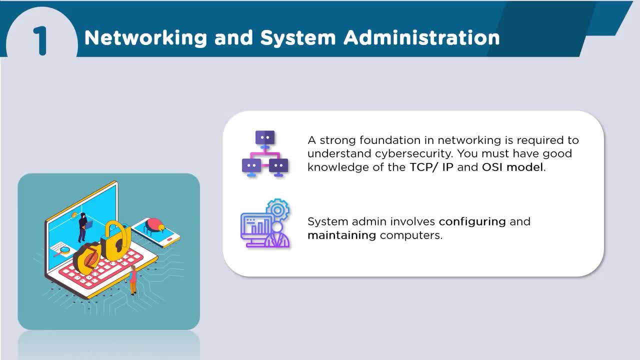 If you think about it, all of us are sysadmins at some level. System administration is all about configuring and maintaining computers. You must be curious to know every aspect of system administration. You must be aware of all the features and settings of your computer and play around a bit. 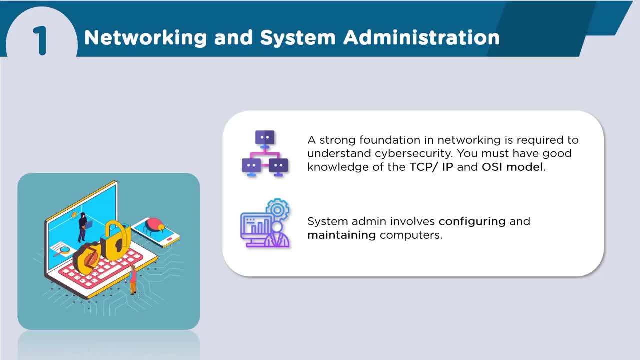 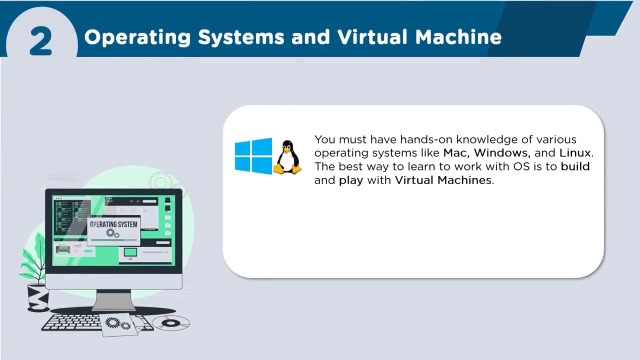 Carry out a trial and error method and give yourself small tasks like recovering deleted files or monitoring old viruses on a VM. Explore new techniques, put them into use and expand your knowledge. Let us now move on to our second skill: Knowledge of Operating Systems and Virtual Machines. 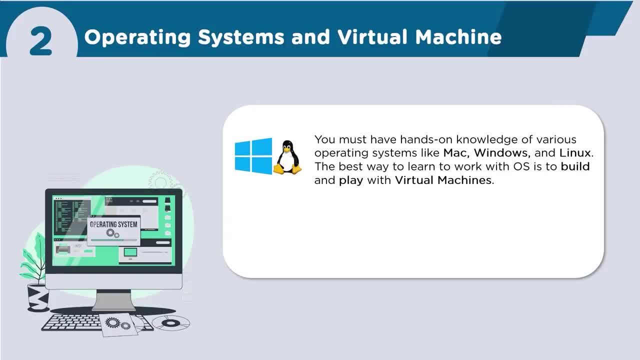 To become a cybersecurity professional, you need to have a strong knowledge of operating environments such as Windows, Linux and MacOS. Cybersecurity professionals largely use Linux and it comes with several tools To learn operating systems, go ahead and set up and use virtual machines, that is, VMs. 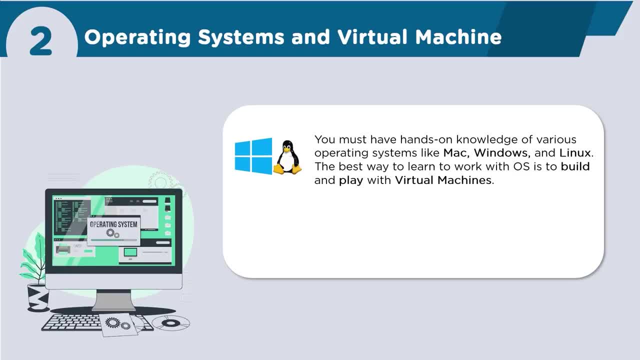 and play around with them. This will help you gain hands-on experience As a cybersecurity expert. you should be comfortable working on any OS. VMs allow you to train and research in an isolated environment and help you maximize your skills. The next point to remember is to know Kali Linux. 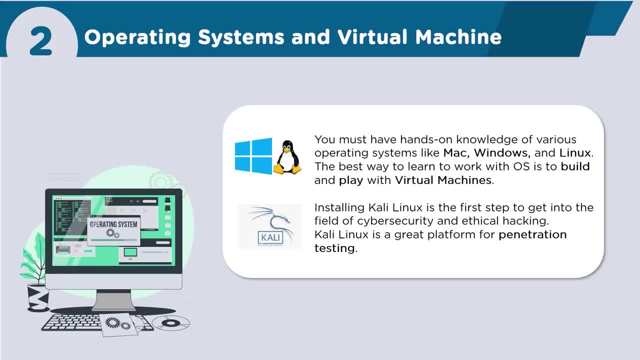 It is the most widely known Linux distribution for ethical hacking and penetration testing. It comes with several hundred tools related to penetration testing, malware analysis, security research, computer forensics and so on. Kali contains several projects and you can learn a lot. 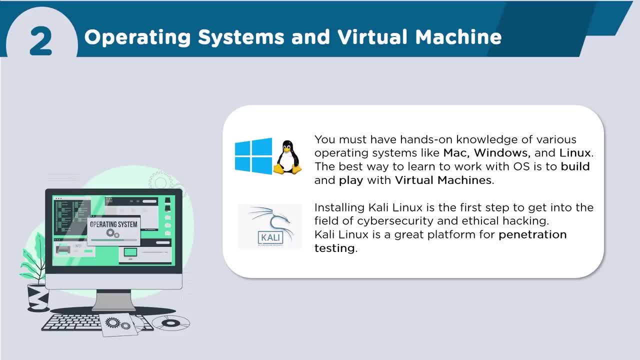 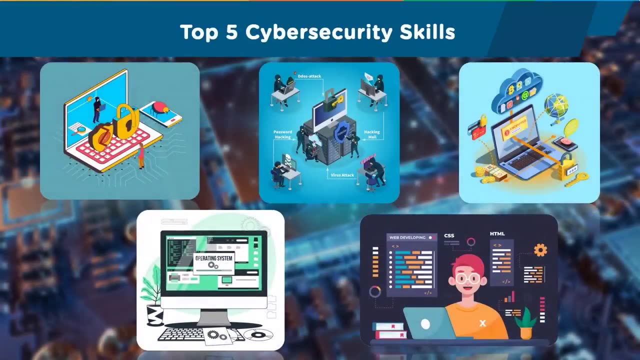 Another good thing about Kali is that it is free to use. So what are you waiting for? Download and start right away. Remember that Linux is the backbone of cybersecurity and a commonly asked topic for cybersecurity interviews, especially for pentesting roles. Moving on to our third skill, 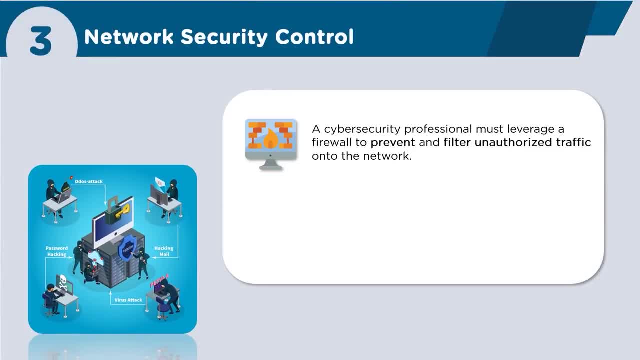 Our third skill is Network Security Control. It is another basic skill that every cybersecurity professional should have. Network Security Control refers to the different measures which are employed to enhance the security of a network. It is simple: you can only safeguard your network if you know how it works. 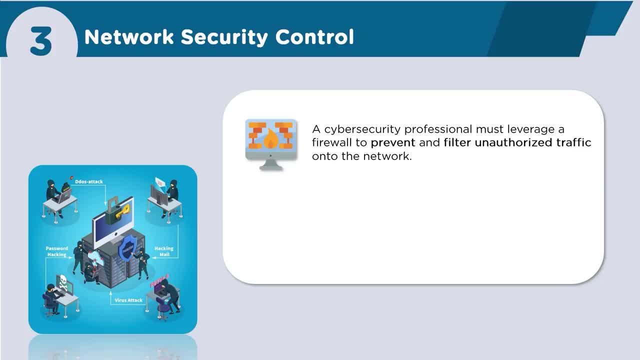 how routers, firewalls and other devices work. A firewall is a hardware or software that blocks incoming or outgoing traffic from the internet to your computer. Firewalls are required to secure a network. A cyber security expert is required. A cyber security expert must be capable of filtering and preventing unauthorized traffic from the network. 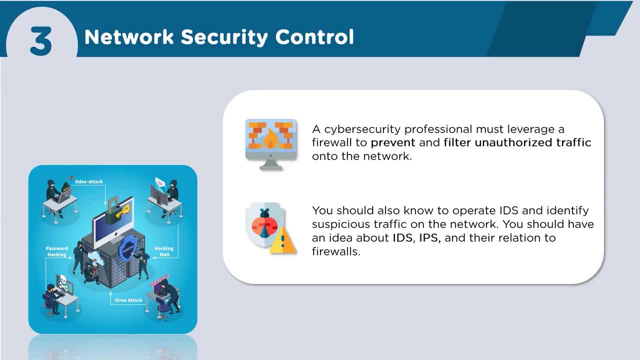 In addition, you must know about the severance of Ruby dengan security device detection systems, buttons of protection and remote remote access. After you are done with this, can you install the security京 system. IDS is designed to detect unauthorized access to a system. It is used together with a. 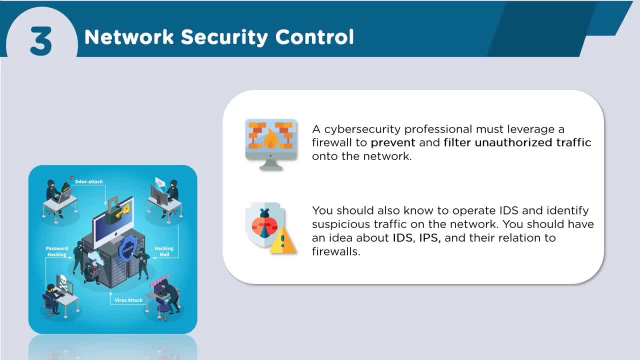 firewall and a router. You should be able to operate the IDS and recognize any security policy violations and malicious traffic on the network. As many of you may have used, a VPN is a connection between a VPN server and a VPN client. It is a secure tunnel across the. 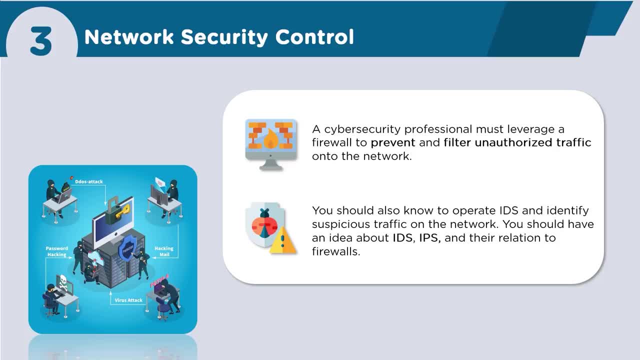 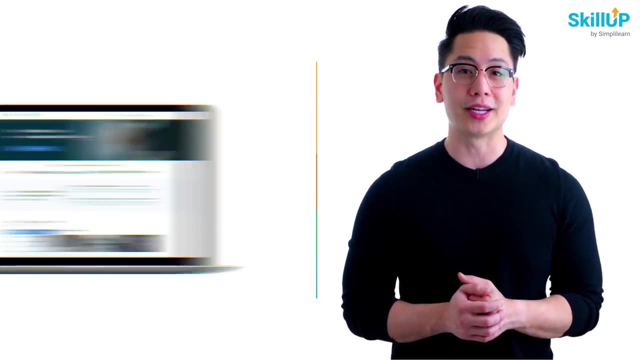 internet. Moving on next up, we have an interesting skill. Any idea what that is? If yes, pause and leave a comment as to what you think the next skill will be. If getting your learning started is half the battle, what if you could do that for free? Visit SkillUp by SimplyLearn. Click on the. 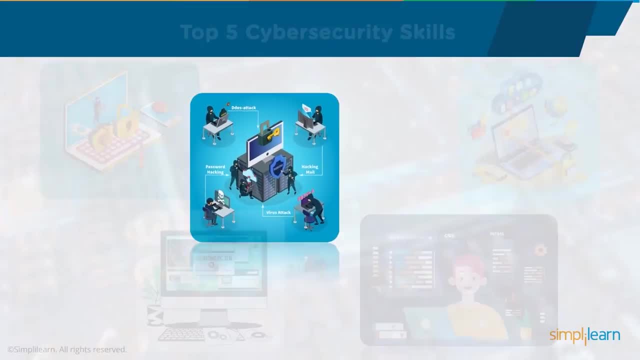 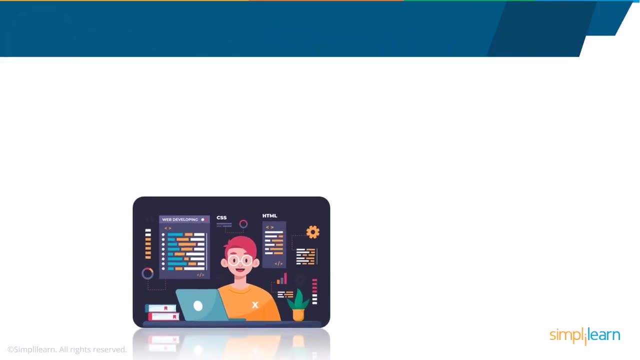 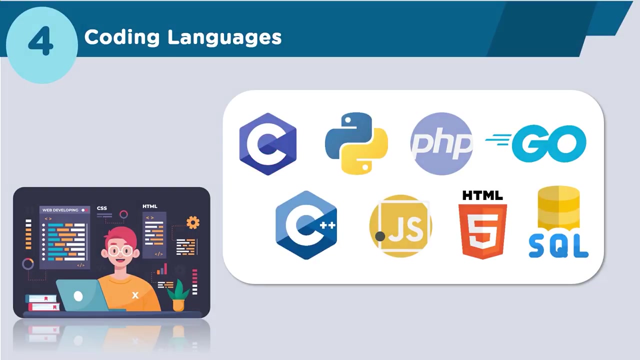 link in the description to know more. And before we jump into this skill, if you find this video interesting, make sure to give it a thumbs up. Fourth skill on our list is the skill of the internet. So you might be wondering if coding is really required to become a cybersecurity professional. 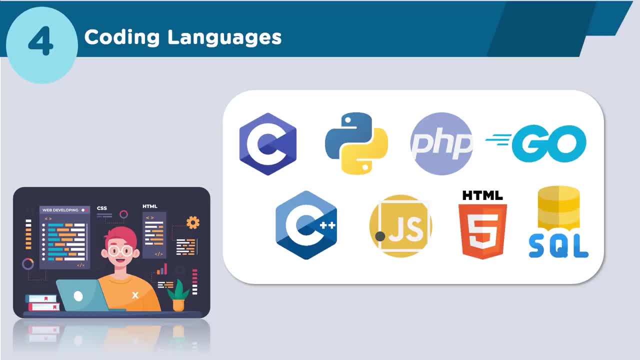 Well, it is true that not all cybersecurity professionals have or need coding skills. However, having zero coding knowledge may limit your opportunities in the future. Knowing a couple of programming languages will help you identify the plan behind an attack and defend against deadly hacking techniques. So, as seen on your screens, these are the 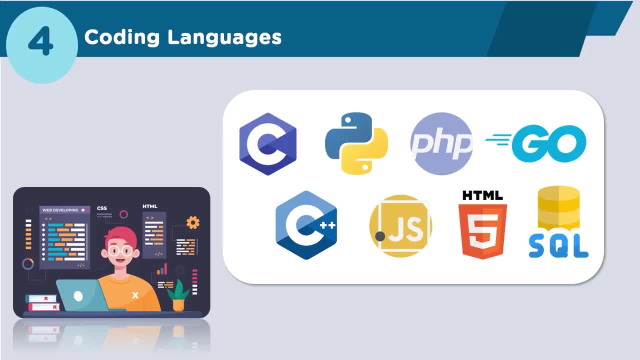 best programming languages to learn to make your life easier. But maybe you are a hands-on wonderer and probably wish this would become a first for you as well. Obviously, some parameters on these three skills are not totaling, so I hope you have to learn to plan ahead for your cybersecurity career. 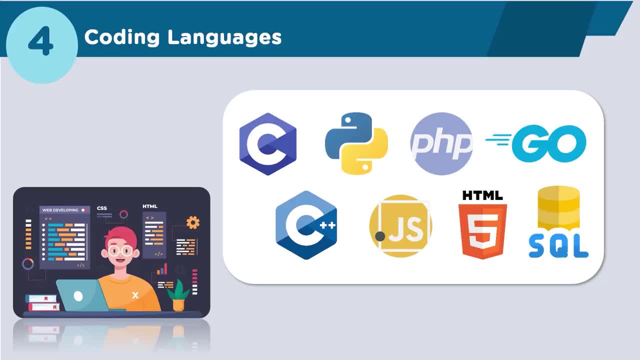 We have C and C++. The C programming language is the backbone of most operating systems. C and C++ are low-level programming languages that you need to know as a cybersecurity professional. On the other hand, Python is a high level programming language that is becoming popular. 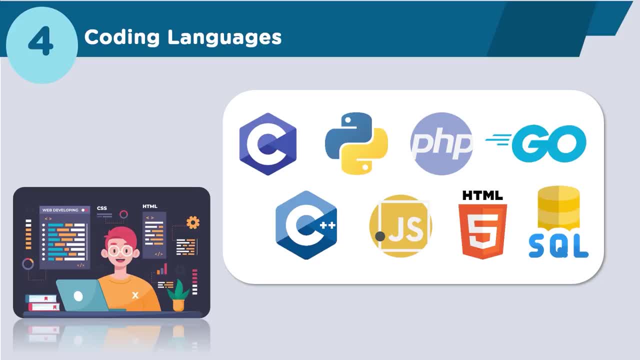 among cybersecurity experts today. Knowing Python will give you an upper hand in your career. It will help you identify and fix vulnerabilities. Super V- outer words, calculating, super ~~- has confirm you've got these upper hand in your career. Your cybersecurity is genuine and você sabe que fazem um melhorы. 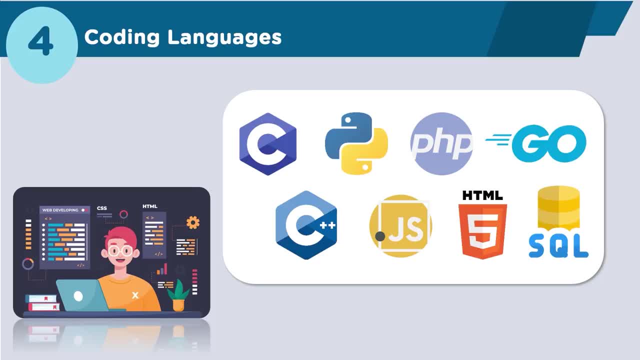 Javascript is another high-level programming language that adds interactivity to web pages. A good advantage of knowing Javascript is that you can prevent cross-site scripting attacks from occurring, As in these attacks, the attacker implants malicious code in a web application Speaking of PHP. because most of the websites are created using PHP, learning it will help. 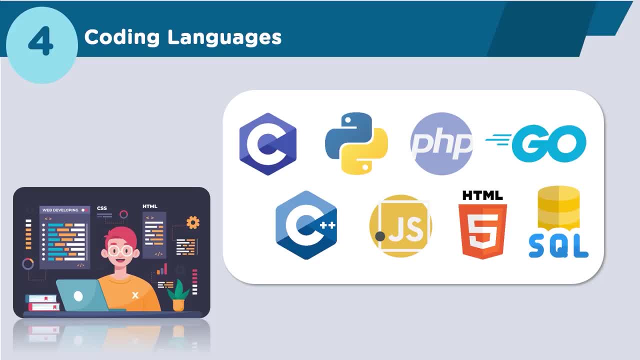 you defend against intruders. Similarly, HTML is another language cybersecurity professionals should understand, as most websites use it and it is one of the easiest languages to learn. Another programming language that you can use is Golang. It is great for cryptography. 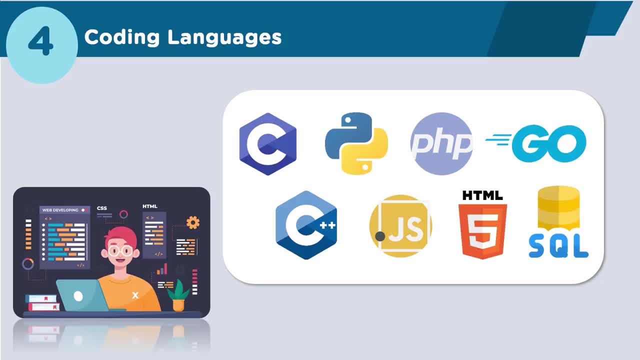 You can solve various cybersecurity problems with it. Then we have SQL, that is, Structured Query Language. Attackers use this language to damage the stored data. One such example is the SQL injection attack. Hence, having a good understanding of SQL will be highly beneficial. 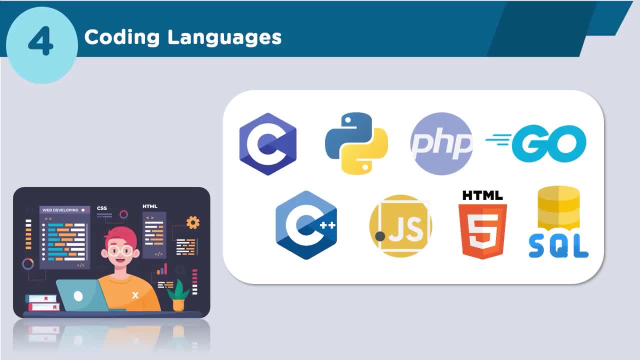 Another point we'd like to highlight is to have knowledge of assembly language. This will help you become a cybersecurity engineer. Assembly will help you understand how malware functions and thereby help you defend against it. In the cybersecurity domain, you can't just lock into a single language and hence it. 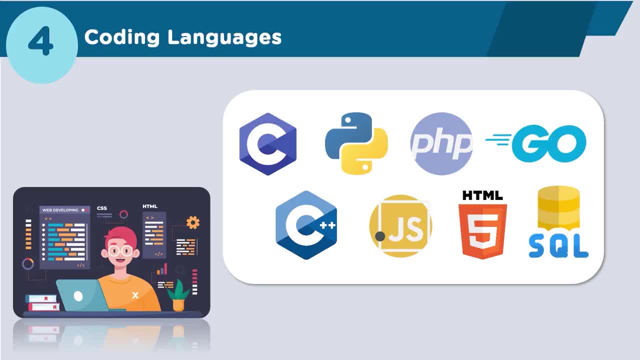 is advised that you're acquainted with a couple of them. You can also do a crash course with these languages and learn them. Hence determine the best programming language for your cybersecurity role and get familiar with the basics. Moving on, our fifth skill on the list is Cloud Security. 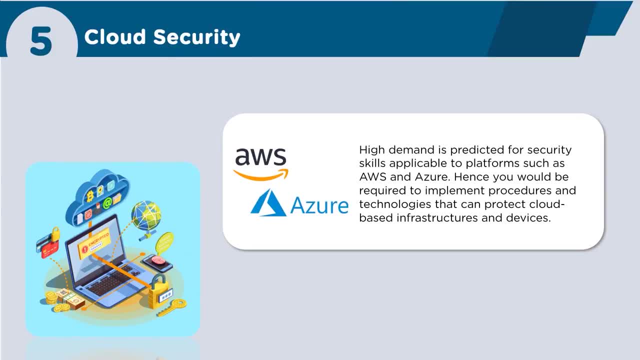 There is a growing demand for cybersecurity professionals with cloud security skills in the coming years. Companies are on the look out for professionals with security skills applicable to public and hybrid cloud platforms such as Amazon Web Services and Azure. More organizations look to cloud infrastructure to store data and run applications. 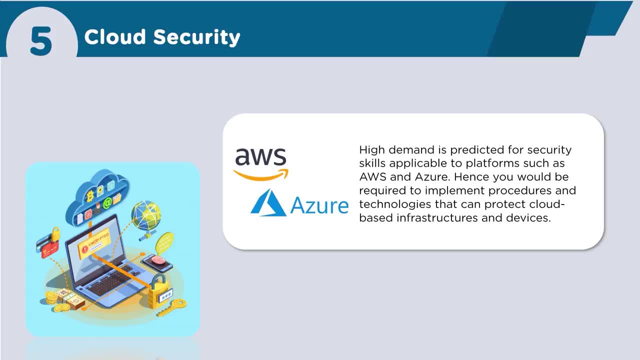 This includes the implementation of policies and technologies that protect cloud-based systems and devices. Just like application development security, cloud security is also a key part of the cloud security ecosystem. Cloud security also involves building secure systems from the start. Companies want professionals who can manage the cloud security tools to identify and prevent. 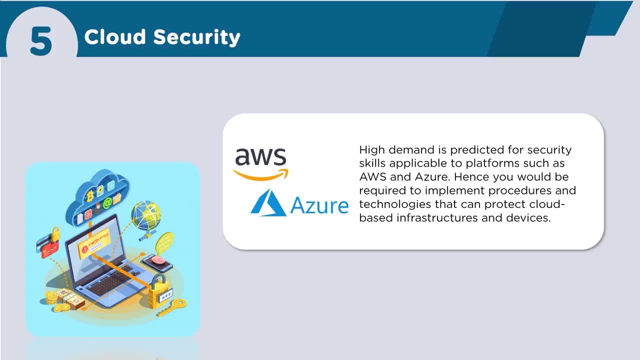 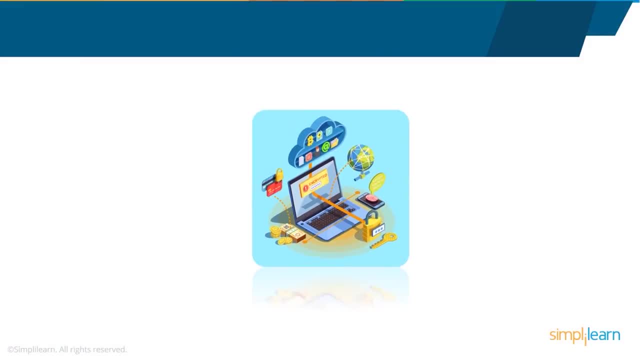 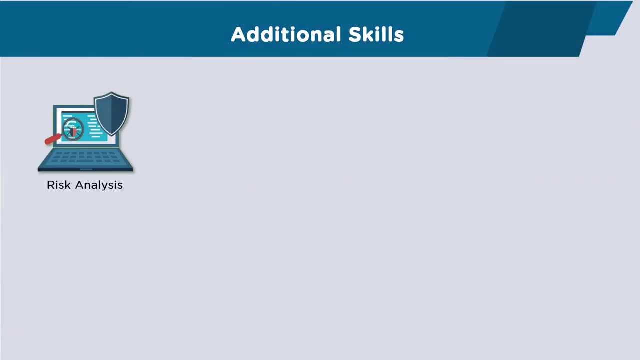 any cloud breaches. People with experience and knowledge in managing big platforms such as Microsoft Azure, AWS and the GCP are in high demand. Now that we have seen the top five cybersecurity skills, let us go through a set of additional skills that can help you get into the cybersecurity field. Remember that to become a successful cybersecurity expert, you must have the following skills. First of all, you need to know how to use the cloud. Second of all, you need to know how to use the cloud. Third of all, you need to know how to use the cloud. Fourth of all, you need to know how to use the cloud. Half of all of you know that you need to know how to utilize the cloud. Fifth, you need to know how to use the cloud And the third challenge is that you need to know how to use it effectively and efficiently. 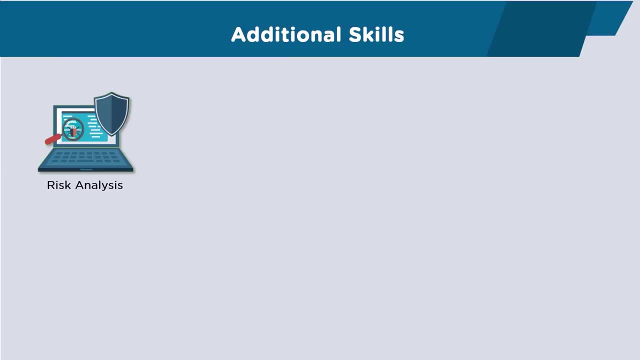 So an example of an additional build over cloud security is risk analysis. Identify risk before your arrival is a great skill. Cybersecurity professionals are required to identify, manage and mitigate risks. Risk management is a skill set that is going to be highly in demand in the coming years. 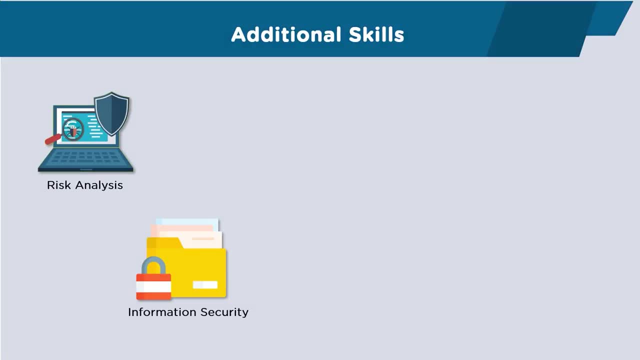 The risk analysisAKE sure it is well documented and well coordinated so they are understood for collection of information. Let's look at information security. First of all, we need to understand how leverage this says on how to handle the risk access. Here in-demand skills are authentication, authorization, malware analysis and data recovery. 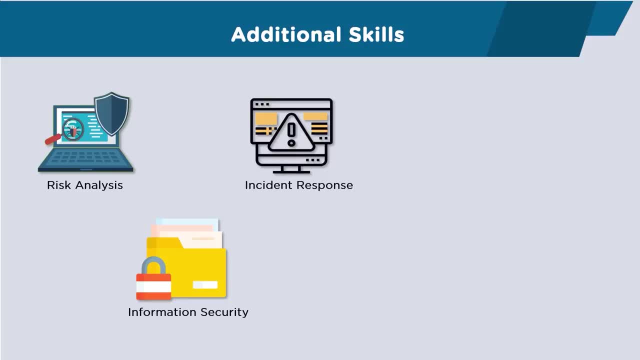 Next on our list is security incident handling and response. As a cybersecurity expert, you must be prepared to handle any forthcoming threat of violating an organization's security policy. By following an updated incident response plan, your team can proactively protect your data and minimize the damages. In security incident management, you are required to identify: 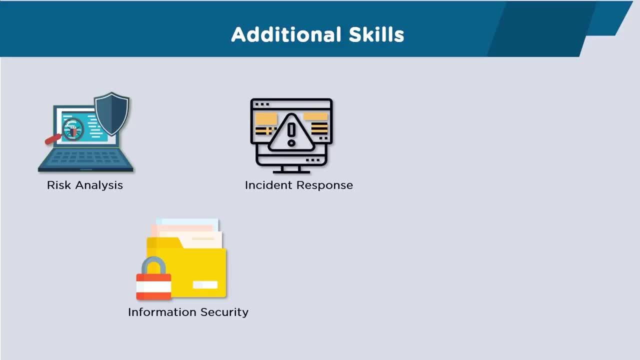 manage, record and analyze security threats in real-time. A security incident can be an active threat, or a successful compromise of data or an attempted intrusion. It can also be incidents like DDoS attacks, phishing, APTs, ransomware and many more. Another important pointer is that, as a 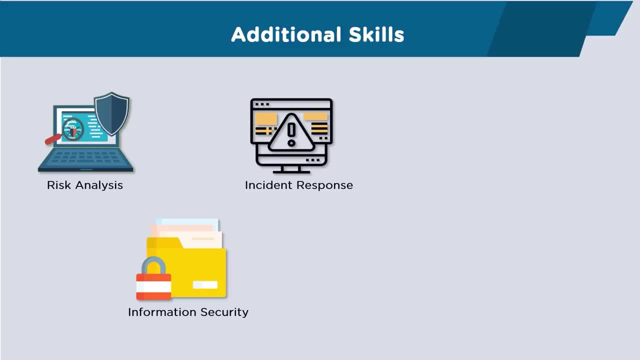 security practitioner, you must also manage and analyze the security information and event management. Moving on, we have security audit. Security auditing is an internal check that is carried out to find flaws in the organization's information system. You must be able to conduct a review of 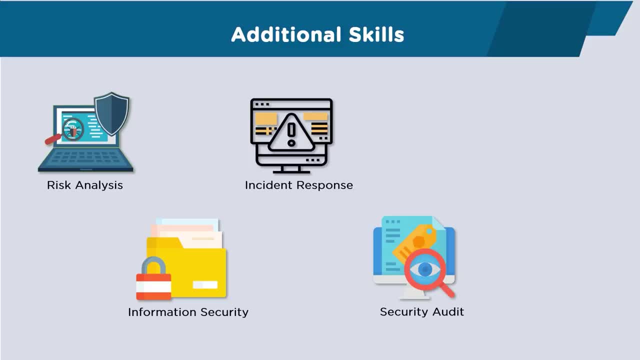 the organization's adherence to regulatory guidelines. Security, audit and compliance knowledge are very crucial, as any mistake of regulatory compliance could lead to hefty penalties. Soon organizations will need people who are more familiar with the various data privacy rules and regulations. For example, if you have a security audit, you must be able to. 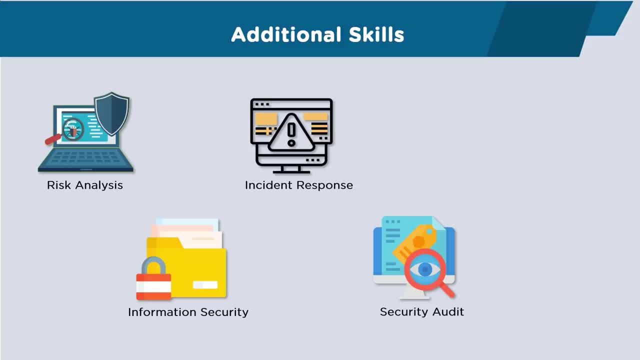 see regulations. If you are good at paperwork, you can capitalize on this skill. Companies will need people who can understand what paperwork to file and which security protocols to use to comply with the regulations. Finally, we have laws and regulations- an often overlooked cybersecurity. 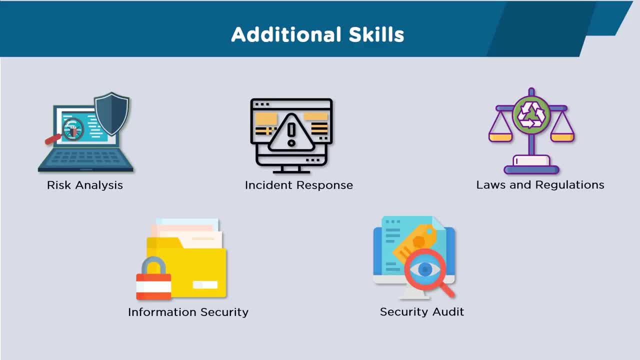 aspect. There are several cybersecurity laws and regulations, and if you break these laws- intentionally or not, it doesn't matter, as you will still be charged. These laws define how you can use the internet, and it also defines how people can use the internet to do things like 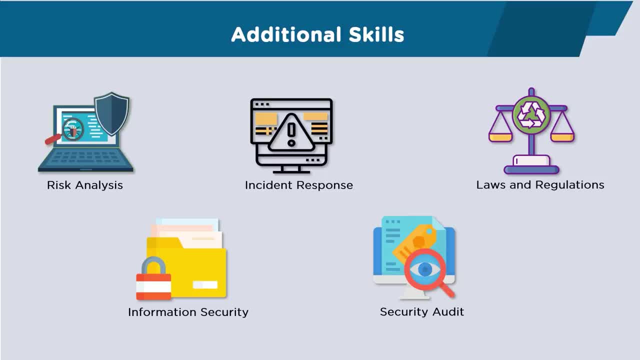 protecting themselves and protecting themselves from being victims of cybercrimes. Knowing these laws and regulations and following the best practice will make you ethical at your job and this will, in turn, be good for your organization. So those were our list of additional skills. 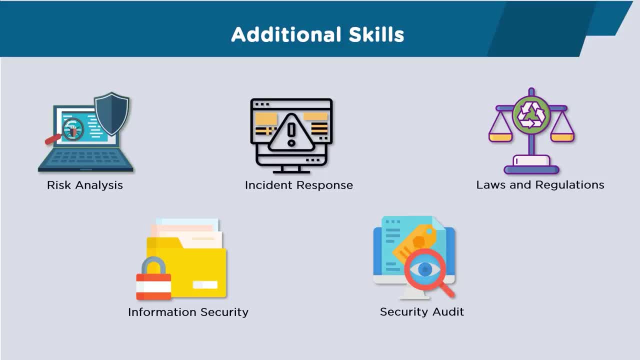 Apart from these, make sure you stay updated with new hacks and learn new tools, as cybersecurity is ever evolving. Another important skill apart from these technical skills is your soft skills. Having a set of good soft skills will help you bag your dream job. We have a video on the top 5 soft skills that will help you grow in your career. 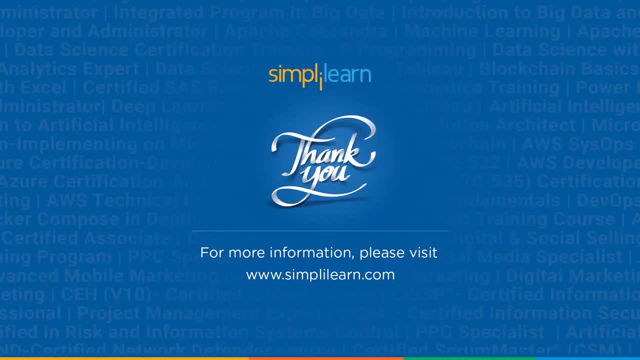 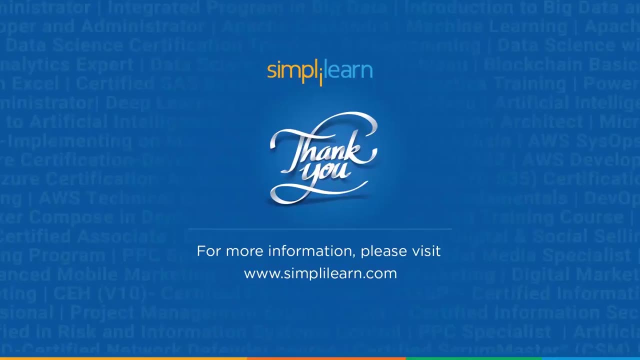 Do watch that and incorporate those skills as well. So with that we come to the end of this video on the top 5 cybersecurity skills. Do you agree with our list? Think we missed anything important? Do let us know in the comment section below. Thank you so much for being here and do watch. 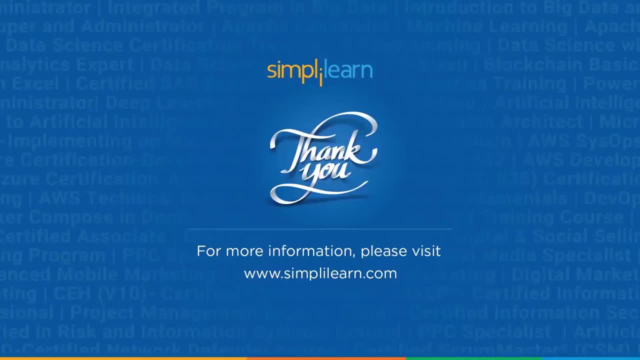 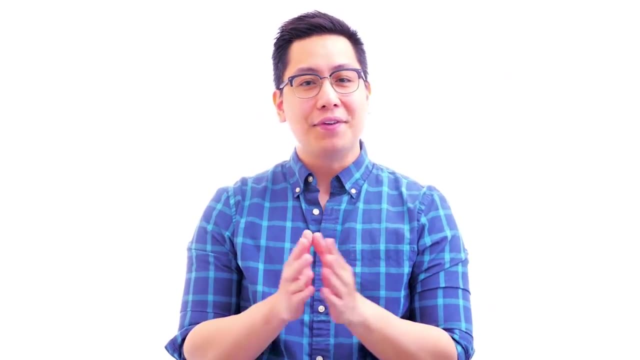 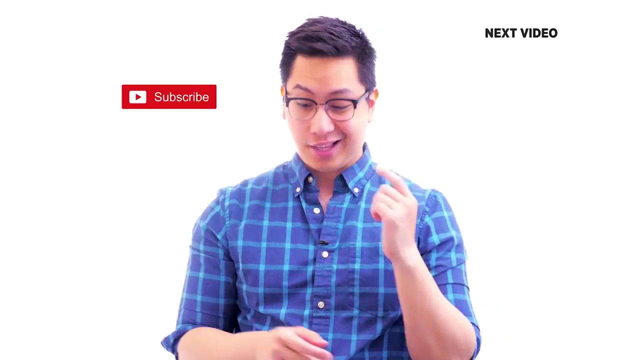 out for more videos from us. Until then, keep learning and stay tuned. to Simply Learn, Like this video. subscribe to the Simply Learn YouTube channel and click here to watch similar videos. To nerd up and get certified: click here.